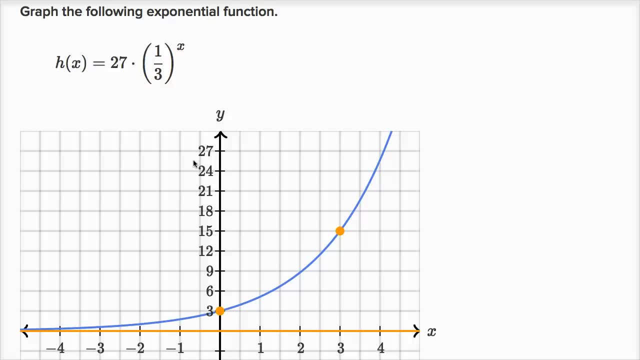 This is from the graph basic exponential functions on Khan Academy. They ask us graph the following exponential function And they give us the function. h of x is equal to 27 times 1, 3rd to the x. So our initial value is 27 and 1: 3rd is our common ratio. 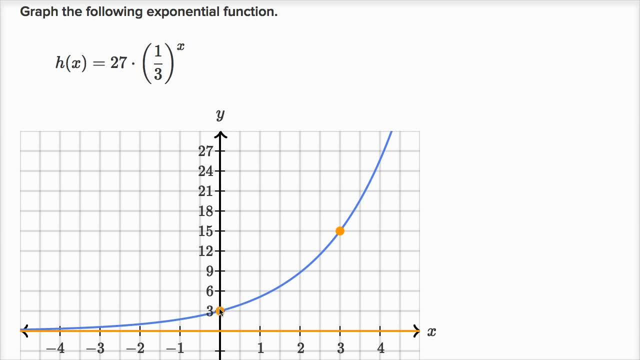 It's written in kind of standard exponential form And they give us this little graphing tool where we can define these two points and we can also define, we can define a horizontal asymptote to construct our function. And these three things are enough to define. 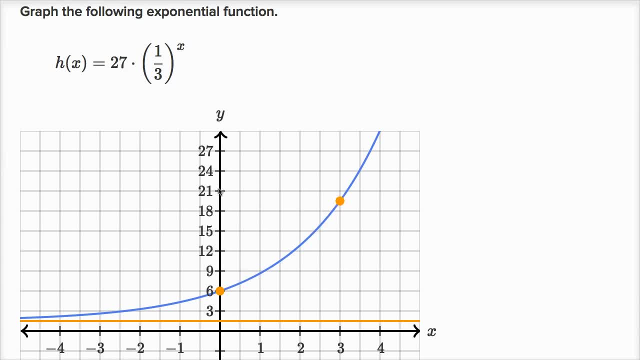 to graph an exponential if we know that it is an exponential function. So let's think about it a little bit. So the easiest thing that I could think of is: well, let's think about its initial value. Its initial value is going to be when x equals zero. 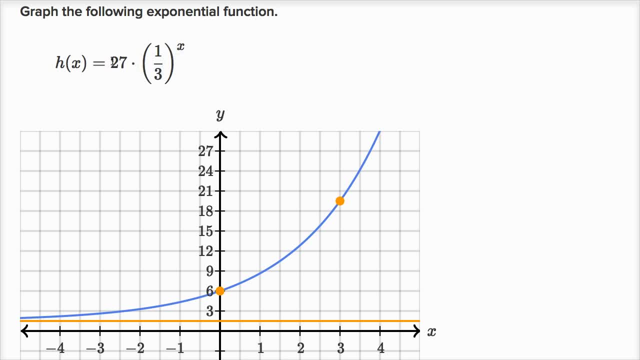 X equals zero. it's 1, 3rd to the zero power, which is just one, And so you're just left with 27 times one, or just 27.. That's why we call this number here when you've written it in this form. 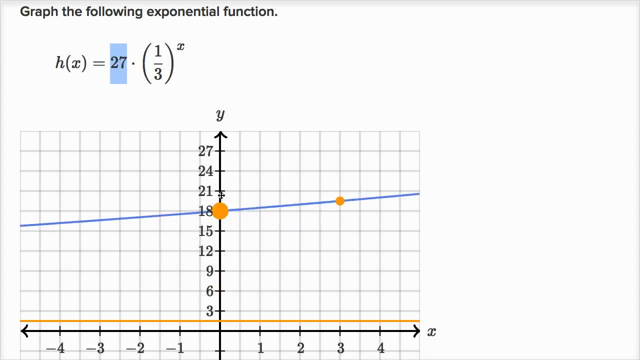 you call this the initial value. So when x is equal to zero, h of x is equal to 27.. And we're graphing: y equals h of x. So now let's graph another point. So let's think about it a little bit. 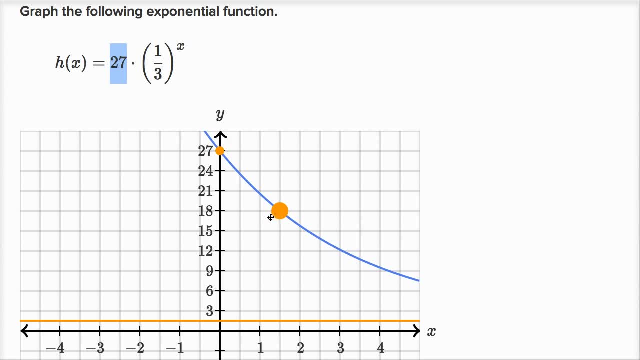 When x is equal to one, when x is equal to one, what is h of x? Well, it's gonna be 1, 3rd to the first power, which is just 1, 3rd, And so 1, 3rd times 27 is gonna be nine. 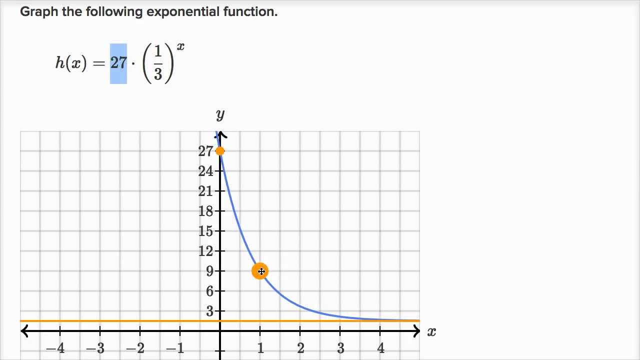 So when x is one, h of one is nine, And we can verify. well, and now let's just think about, let's think about the asymptote. So what's gonna happen here when x becomes really really, really, really, really, really big? 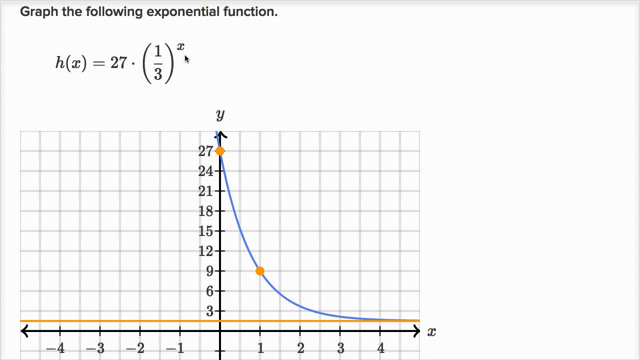 Well, if I take 1, 3rd to like a really large exponent, say to the 10th power or to the 100th power or to the 1000th power, this thing right over here is going to start approaching zero. 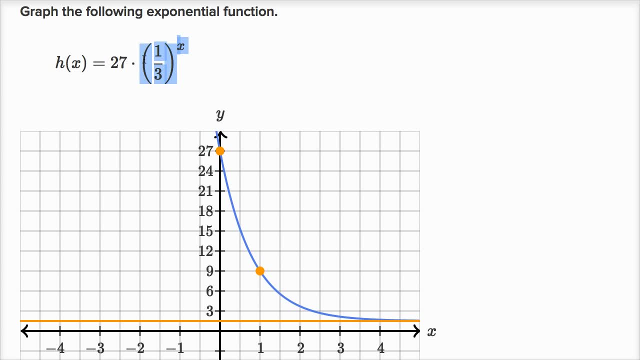 as x becomes much, much, much, much larger, And so something that is approaching zero times 27,. well, that's going to approach zero as well. So we're gonna have a horizontal asymptote at zero, And you can verify that this works for more than. 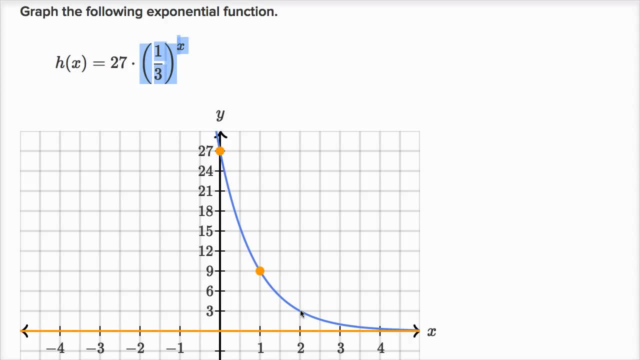 just the two points we thought about. When x is equal to two, this is telling us that the graph y equals h of x goes through the point two comma three, So h of two should be equal to three, And you can verify that that is indeed the case. 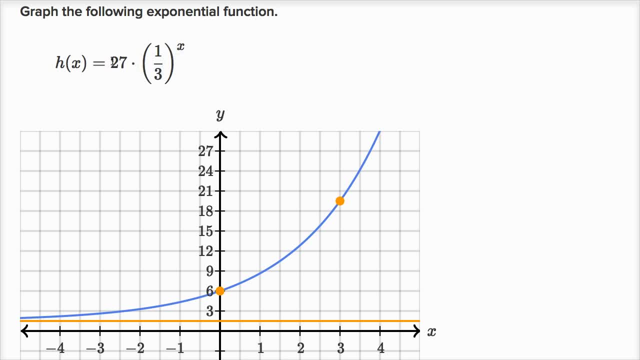 X equals zero. it's 1, 3rd to the zero power, which is just one, And so you're just left with 27 times one, or just 27.. That's why we call this number here when you've written it in this form. 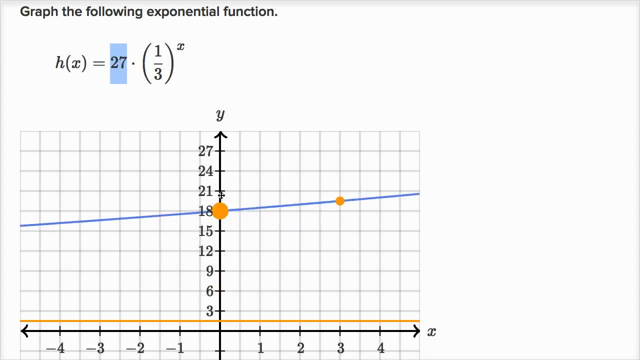 you call this the initial value. So when x is equal to zero, h of x is equal to 27.. And we're graphing: y equals h of x. So now let's graph another point. So let's think about it a little bit. 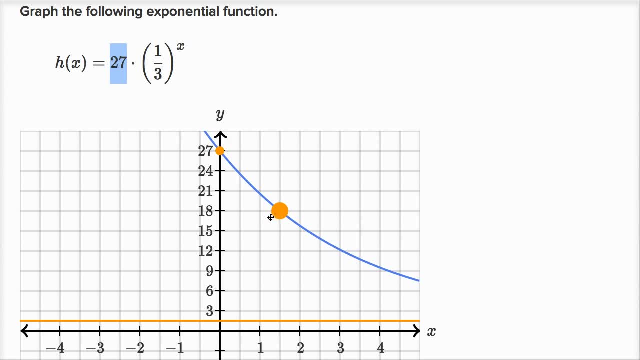 When x is equal to one, when x is equal to one, what is h of x? Well, it's gonna be 1, 3rd to the first power, which is just 1, 3rd, And so 1, 3rd times 27 is gonna be nine. 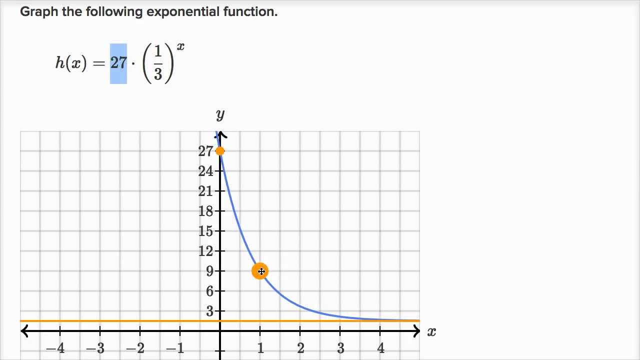 So when x is one, h of one is nine, And we can verify. well, and now let's just think about, let's think about the asymptote. So what's gonna happen here when x becomes really really, really, really, really, really big? 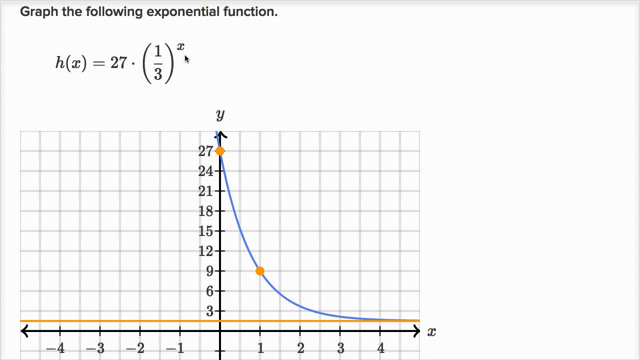 Well, if I take 1, 3rd to like a really large exponent, say to the 10th power or to the 100th power or to the 1000th power, this thing right over here is going to start approaching zero. 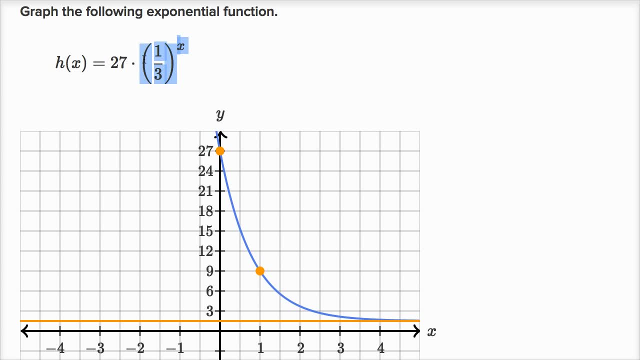 as x becomes much, much, much, much larger, And so something that is approaching zero times 27,. well, that's going to approach zero as well. So we're gonna have a horizontal asymptote at zero, And you can verify that this works for more than. 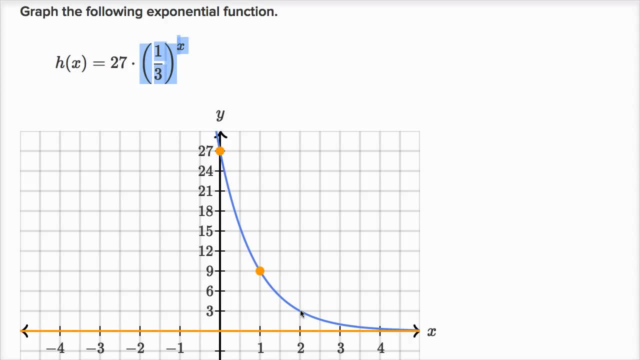 just the two points we thought about. When x is equal to two, this is telling us that the graph y equals h of x goes through the point two comma three, So h of two should be equal to three, And you can verify that that is indeed the case. 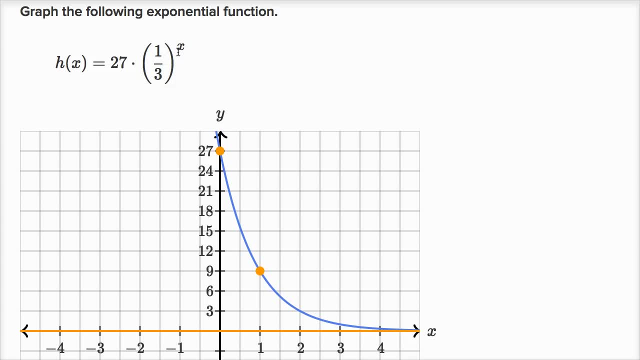 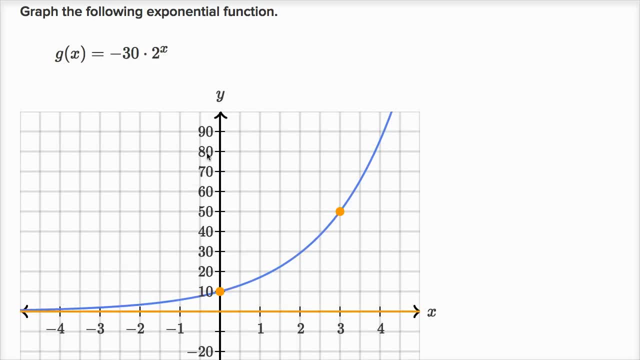 So I feel pretty good about that. Let's do another one of these. So graph the following exponential function: So same logic: When x is zero, the g of zero is just going to, is just going to boil down to that initial value. 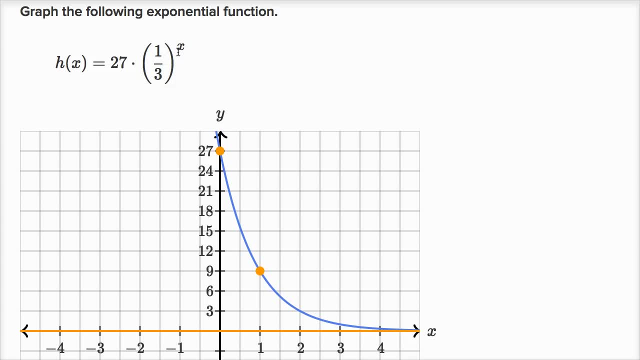 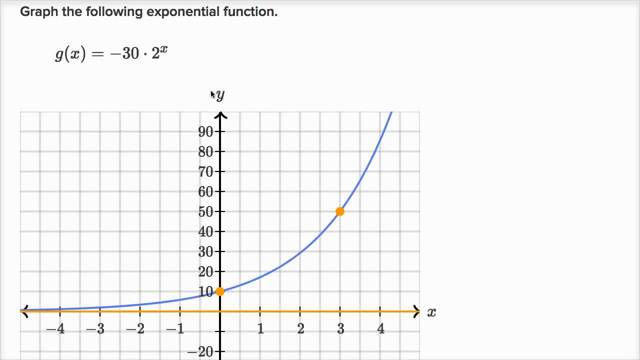 is three, So I feel pretty good about that. Let's do another one of these. So graph the following exponential function: So same logic. When x is zero, the g of zero is just going to boil down to that initial value, And so let me scroll down. 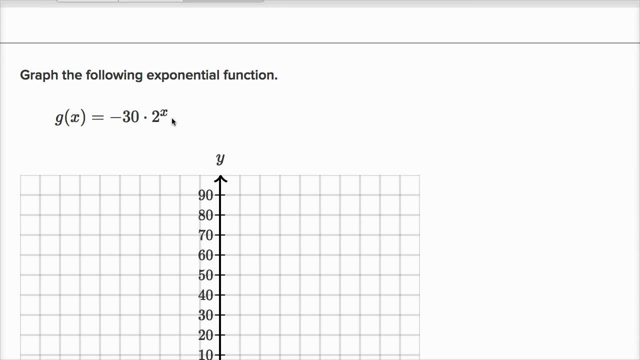 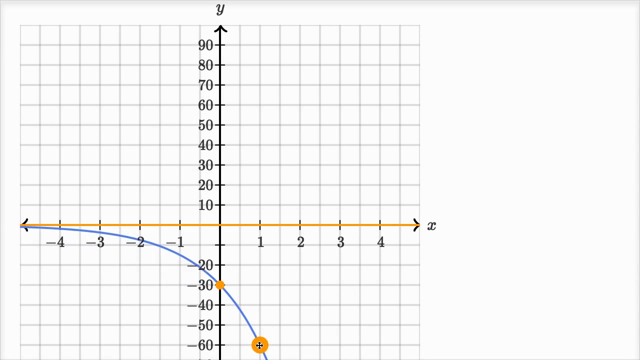 The initial value is negative 30.. And so let's think about when x is equal to one. When x is equal to one, two to the first, power is just two, And so two times negative 30 is negative 60.. When x is equal to one, the value of the graph is negative 60.. 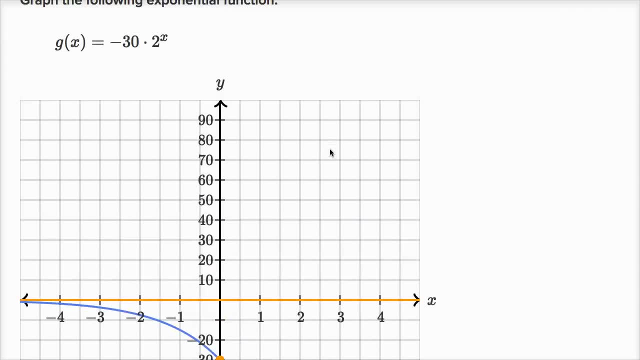 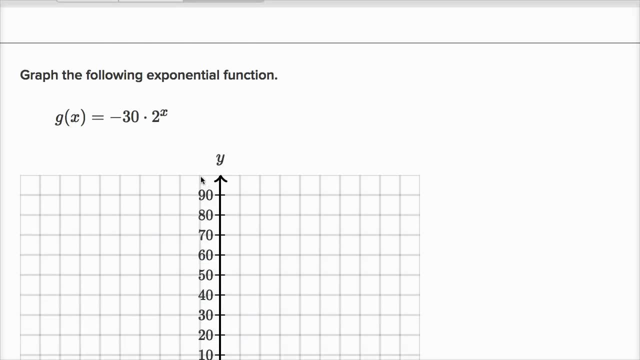 Now let's think about this asymptote, where that should sit. So let's think about what happens when x becomes really, really, really, really, really, really negative. So when x is really negative. so 2 to the negative 1 power is 1 half. 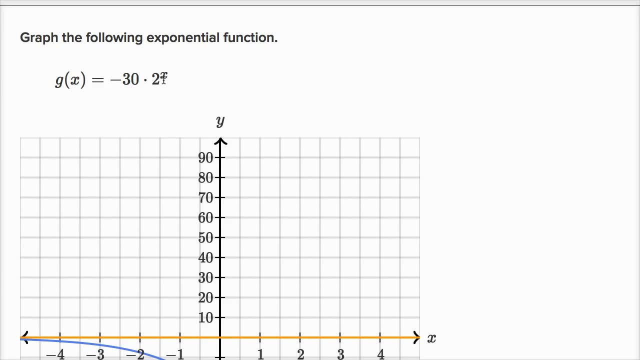 2 to the negative. 2 is 1. fourth. 2 to the negative: 3 is 1- eighth. As you get larger and larger magnitude negative values, or in other words, as x becomes more and more and more negative, 2 to that power is going to approach 0.. 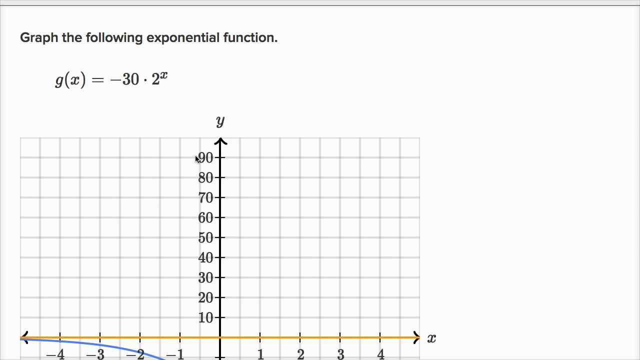 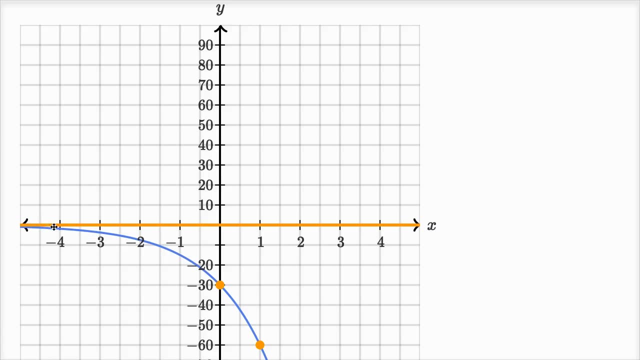 And so negative 30 times, something approaching 0 is going to approach 0. So this asymptote's in the right place, Our horizontal asymptote: as x approaches negative infinity, as we move further and further to the left, the value of the function is going to approach 0. 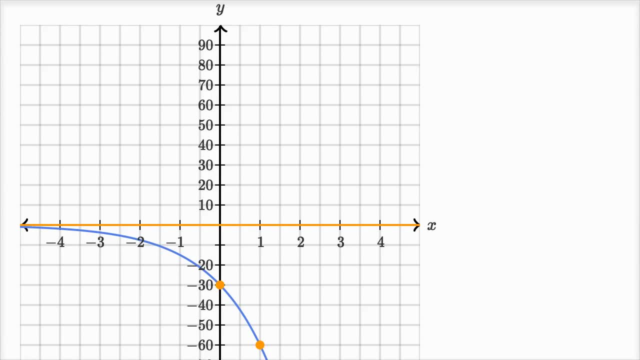 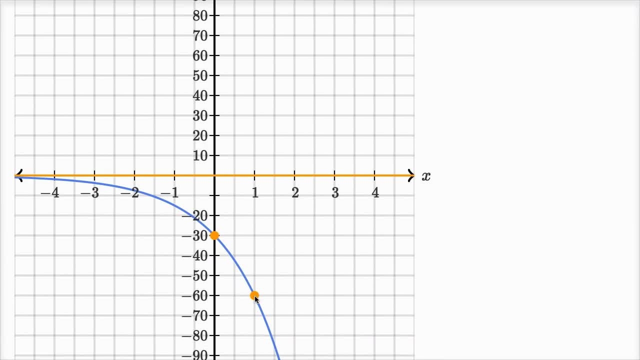 Because we already looked at the initial value and we used that common ratio to find one other point. Hopefully you found that interesting. Introduction. Most rainforests in the world are located in the tropics close to the equator. 57% of all tropical rainforests are found in Latin America. Brazil is home to one-third of all the tropical rainforests in the world, including. the famous Amazon rainforest. Tropical rainforests are hot and humid. Typical temperatures are between 21 and 30 degrees Celsius. Though the average monthly rainfall is 6 centimeters, it has been known to rain up to 5 centimeters in just one hour. Since there is so much rain.